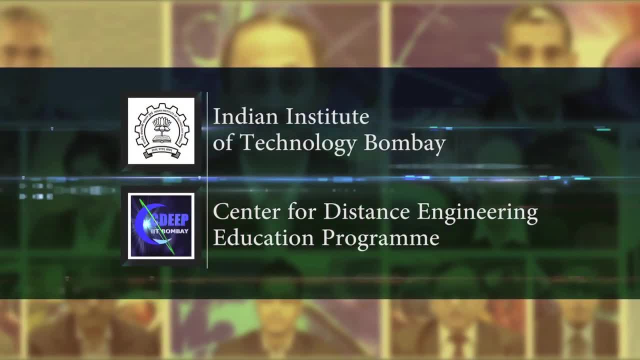 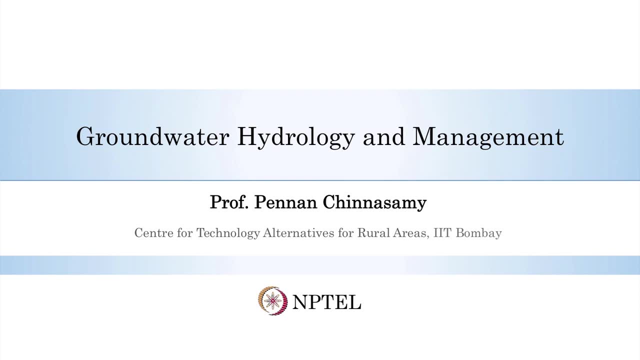 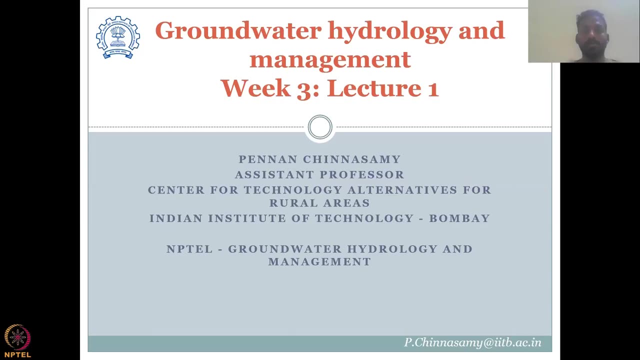 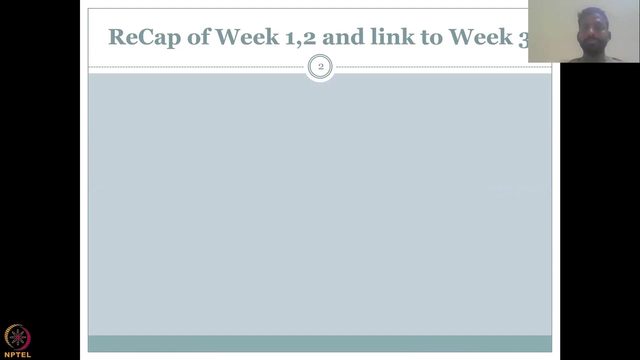 Hello everyone, welcome to NPTEL course on groundwater hydrology and management. This is week 3, lecture 1.. Let's do a quick recap of what we did in week 1 and week 2 and how it is linked to week 3.. So in the week 1, we looked at introduction to groundwater. 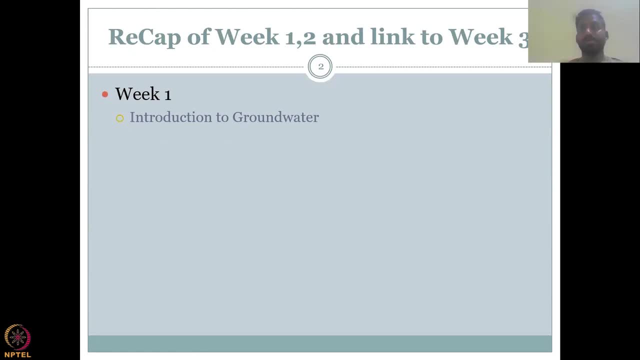 We looked at how groundwater stress is there? what are the uses of groundwater? what do you mean by groundwater from the hydrological cycle, etc. We built it from the understanding of groundwater where it is used more. what are the importances of groundwater? what fields do they sustain and prolong, for example, livelihoods, domestic. 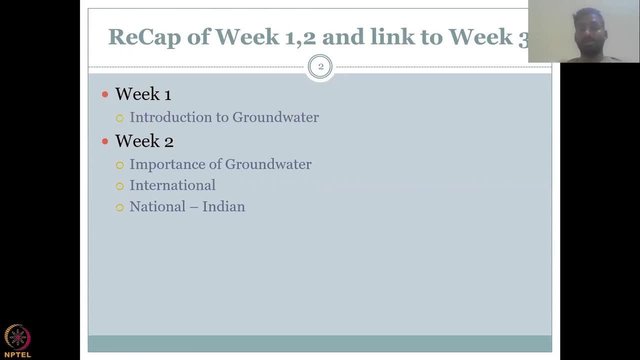 use: agriculture, sanitation, industry, etc. We focused a lot on the international scale. We looked at different countries and countries. We looked at the different continents and saw how groundwater has been used. We also looked at the key segments which use groundwater, especially agriculture and within. 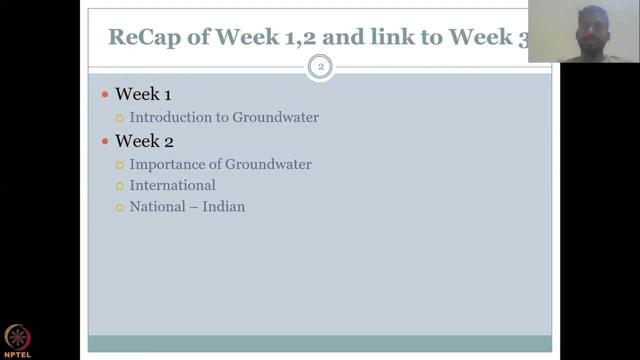 agriculture, we also looked at certain crops. Then, by the end of week 2, we also moved towards the national scale, Indian scale, and we understood that there are a lot of issues in groundwater. Yes, Because in many places groundwater is unsustainably used. 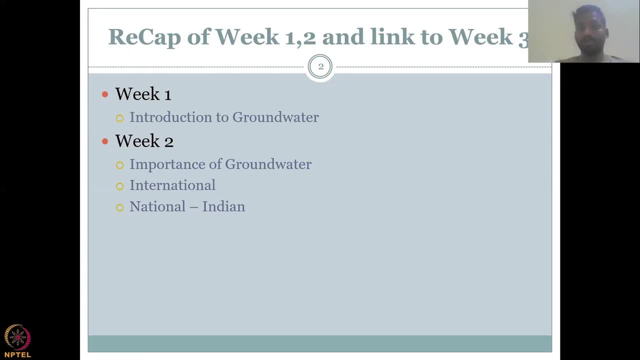 The level of depletion is not sustainable for long term groundwater use And for the fact that India is the leading groundwater extractor in the world, Even though India is not as big as US or China, which are ranked number two and number three in groundwater use. 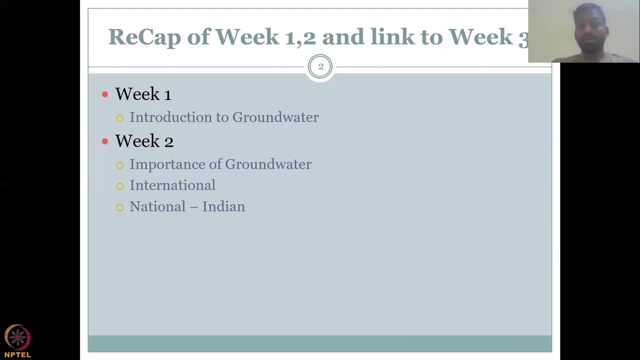 Still our use is much bigger than China and US. In fact, some reports claim that our groundwater use is above the combined use of US and China. So, given the fact that the land is less, the rainfall is not as much the total net rainfall. 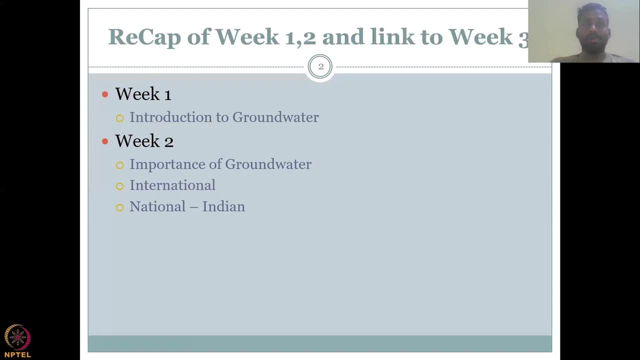 is not as much as in these two countries. it is not right to use so much of groundwater. So the importance now shifts to conservation. We need to conserve groundwater. Before we get into conserving groundwater, we need to know the groundwater hydrology. 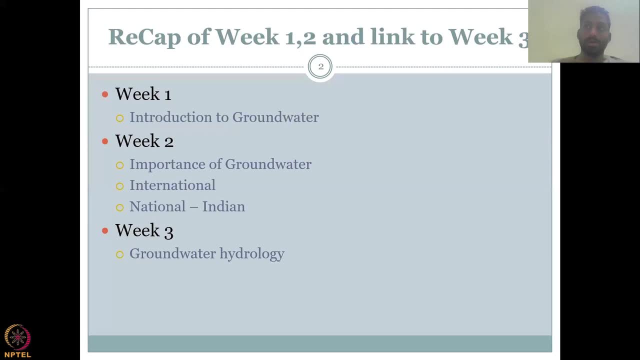 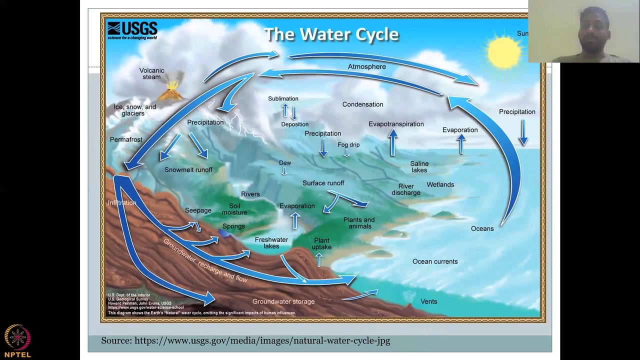 So we have length: week one, week two and slowly transitioning into week three where we look at groundwater hydrology. what does it mean? What are the different components of groundwater hydrology? before that, a just quick, short review of what is hydrology. we know hydrology is the 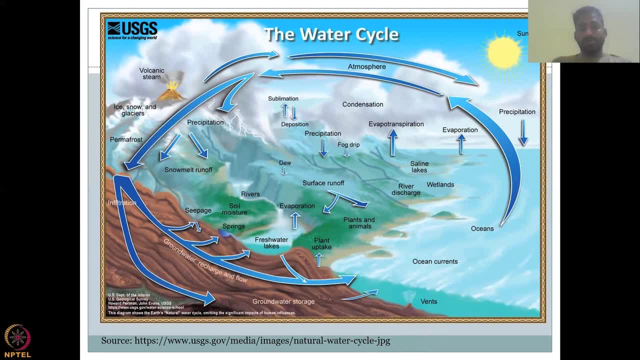 structural movement of water, documenting the movement of water. and the movement of water is given like a hydrological cycle or a water cycle, as this image shows. we've already visited this in week one. i'll just quickly revisit some concepts here and then we'll dive into groundwater hydrology. so even though there are multiple 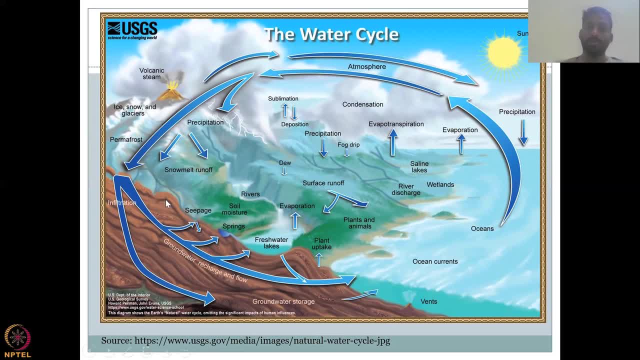 major components in the hydrological cycle. there are a few components that focus on the groundwater. if you could see here the rain or the surface water, let's club all this into surface water. all the water sources like precipitation, snow, melt, sublimation, deposition- um how far would you? rivers, stream, ocean, all of this, let's club it to. 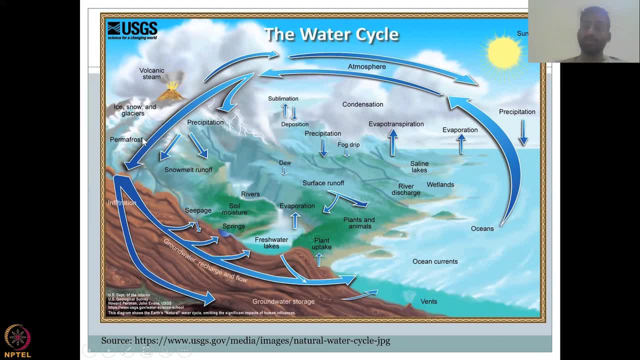 as surface water. And now, when the surface water touches the ground, there is infiltration, percolation and then storage of groundwater in different compartments. Slowly, groundwater moves in and out of the earth's crust. When it moves out, it's called discharge. when it moves back in, 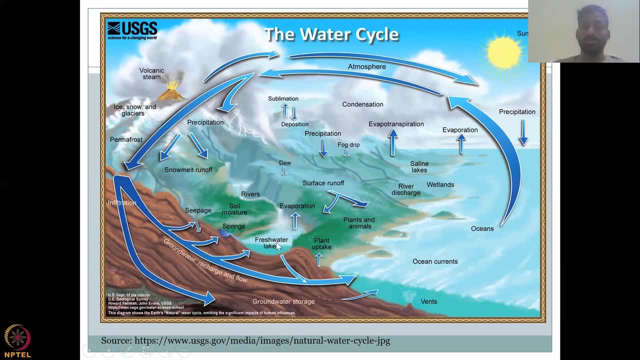 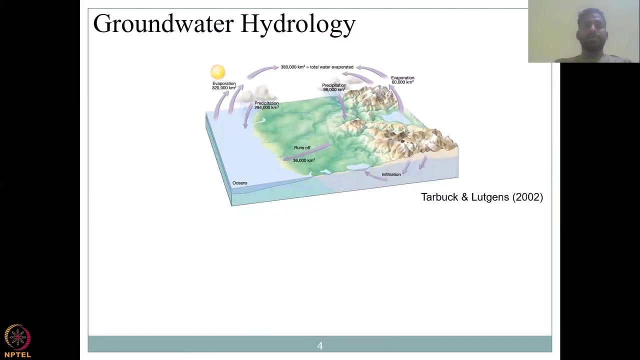 it's called recharge. So you see here it's moving out into the lake and from the lake groundwater comes back in. So the study of groundwater hydrology will look mostly these underground drivers for groundwater movement and that is what constitutes groundwater hydrology. So you could see here that again the hydrological cycle is shown. 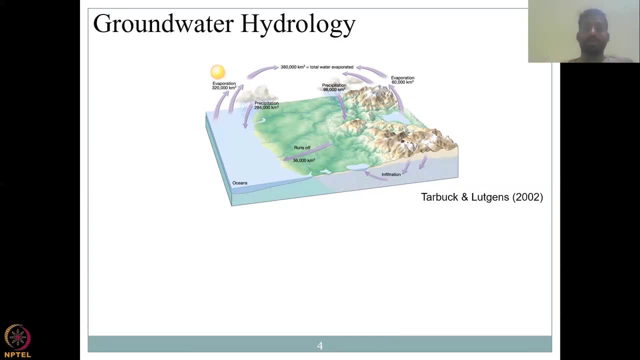 because groundwater hydrology is a part of the overall hydrology, just a segment. When we talk about oceans and lakes, yes, it is part of a hydrological cycle. We cannot totally take it out right. It is some groundwater is given in some snow melt, and so the unit is hydrology or water cycle. 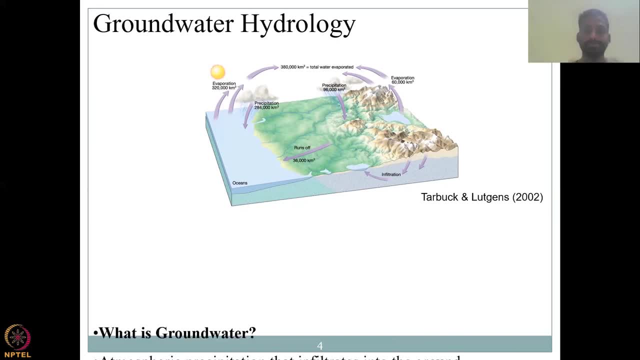 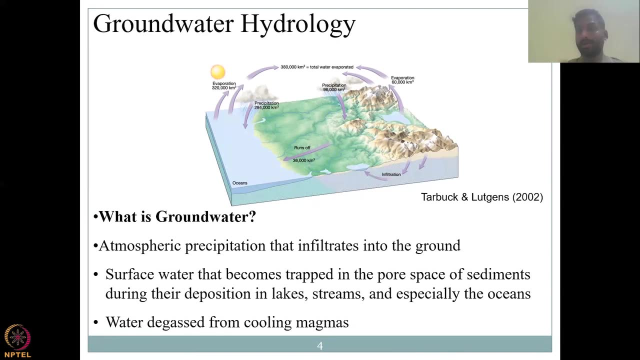 and then in that one part is groundwater, hydrology. So what is groundwater? Let's define groundwater to be more specific and where it comes from. Groundwater comes from the atmospheric precipitation, which is your rainfall or snowfall or dew, from multiple, multiple. 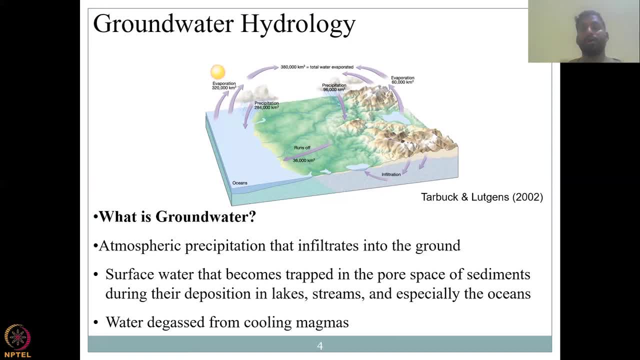 resources for atmospheric precipitation, and once that water infiltrates into the ground, it becomes groundwater. It's the same water, but on the top of the surface it may be called as a river lake and in the atmosphere it may be called as a precipitation: rainfall, dew, humidity, water vapor, anything But. 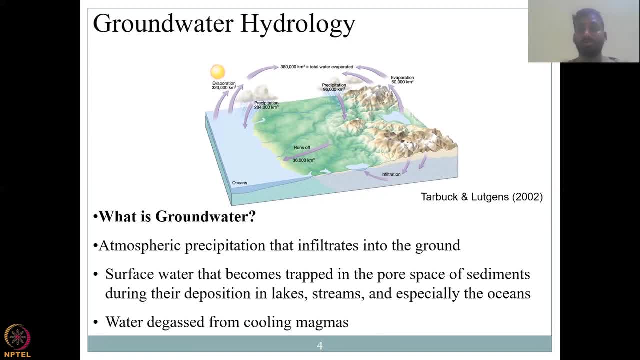 groundwater gets into the ground through infiltration, It is called groundwater. Surface water that becomes trapped in the pore space of sediments during depression etc. can also constitute groundwater. We all know that the plates are moving, the continental plates we call. They are always in motion. You have earthquakes, you have new formation of land and some land submerging. 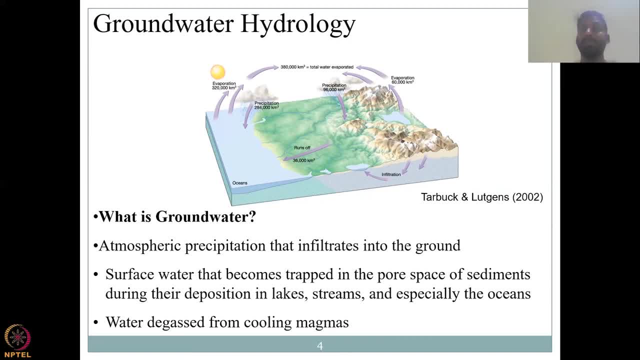 So when the new land forms or when deposition happens, the lakes and rivers carry a lot of sediments and when they get deposited on the surface, sometimes water gets locked right because there's some moisture and then you pile up sediments or a big deposition and 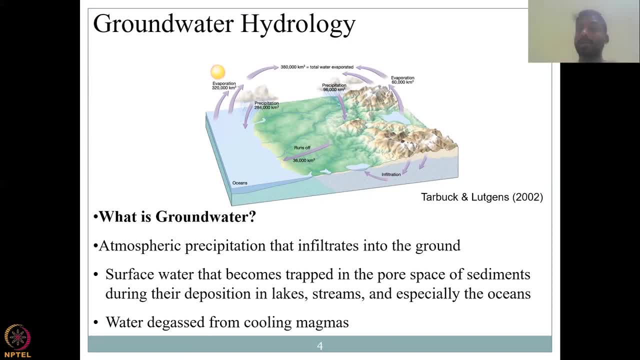 you pile it up, water is trapped underneath and that can also be constructed as a groundwater. Another source of water is throughignon, the chemical reactions that happen underground, mostly by water degas from cooling magmas. So when hot molten lava cools down, there is water degassed from that element and that water has. 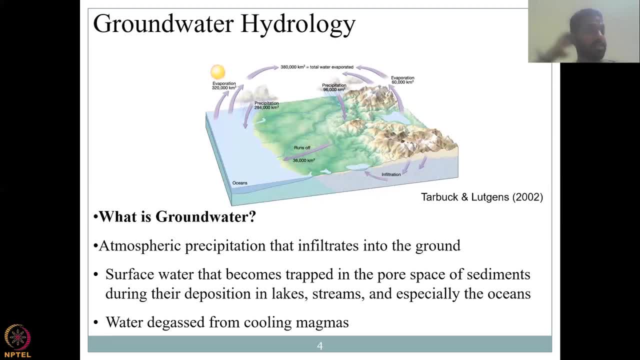 nowhere to go, so it gets trapped. So once these trapped waters get connected, then it starts to move and you have groundwater hydrology. So please understand that it is a part of the overall hydrological cycle and we would focus mostly on the water that is underground. 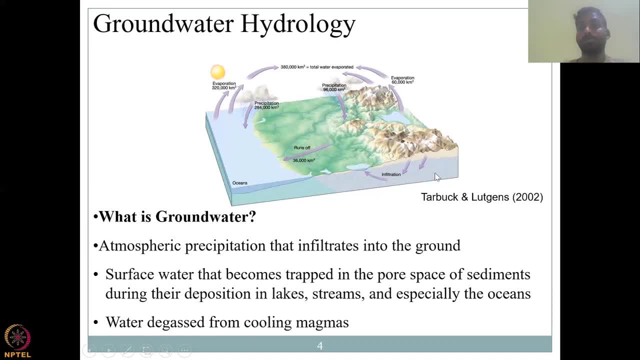 and there are some components of water which are only stored. they are not connected. and if they are not connected, still, they are part of the hydrological cycle but they don't move. So because it is connected, here you could see water moves down your mountains and then goes. 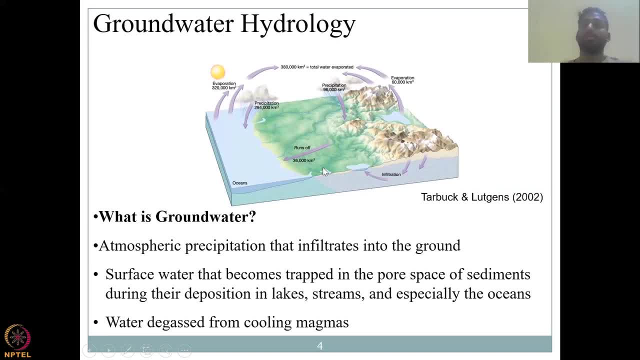 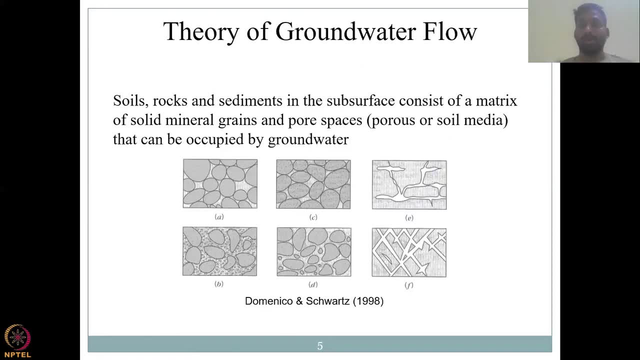 into infiltration and comes up right. There are some water which can just stay there for a long time. Everything constitutes groundwater hydrology. Let's look at the theory of groundwater flow. So the most most basic element for understanding the groundwater flow is to understand where the 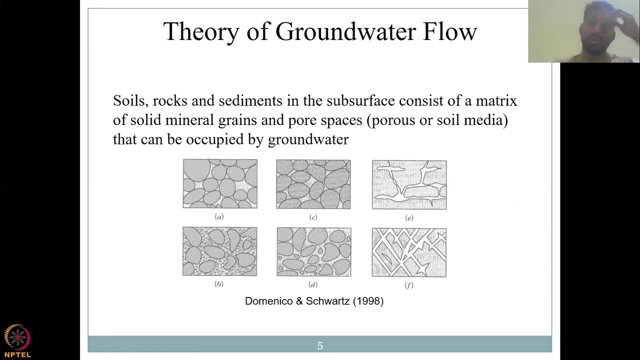 groundwater is going to be stored. So we know groundwater constitutes of different types of water that gets into the ground. but to get into the ground there has to be some space and storage. If it is full solid rock, solid rock water cannot get in right. So there is some space and that would 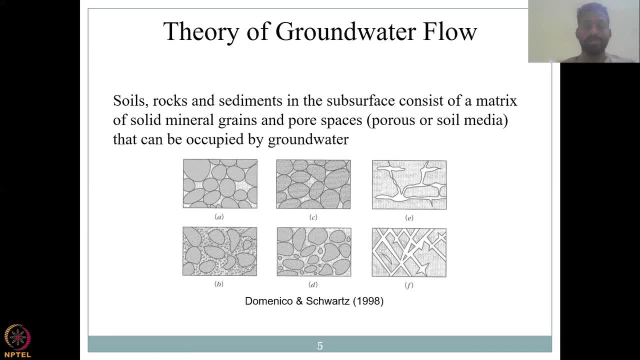 be a very, very important factor for groundwater hydrology. Soils, rocks and sediments in the subsurface and underground ground of a matrix of solid mineral grains and pore spaces have a lot of pore as space. Porous space means a space with a lot of void. 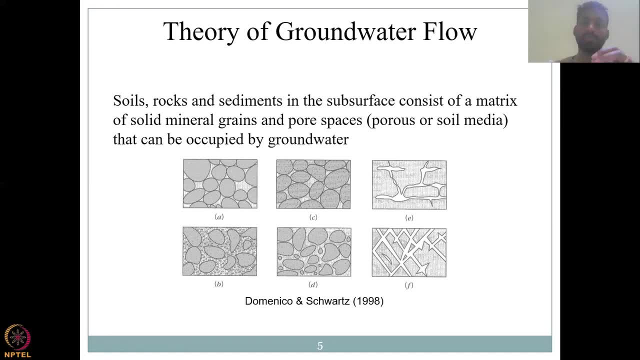 So you cannot store it, or a place where inside the sediment and rock there is no rock and sediment. It's a void, empty place. So they have a lot of these mineral grains and they are structured in a particular manner and because they are structured, there is a possibility of having space. So let's take A, for example. 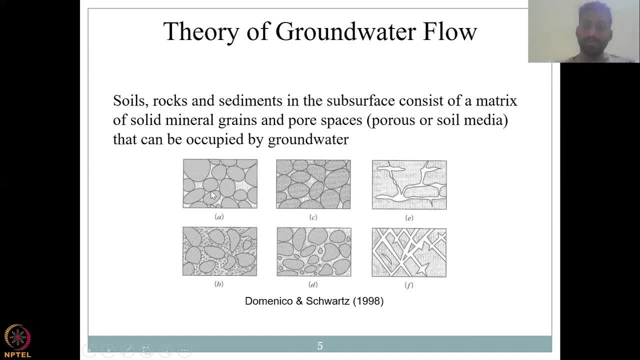 You have round sediment, solid minerals, and there are a range of minerals arranged in a fashion that the bigger elements are there and in between the bigger elements you have smaller elements. but inside that, inside that, there is some space, so you could see there's a big rock material and then you have another space here. right, these spaces? 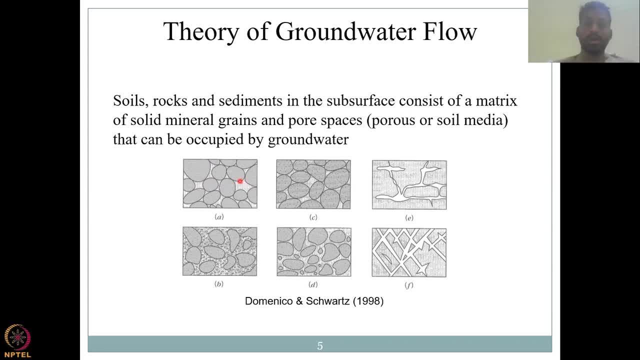 are where the water can be stored. excuse me, then, you have within the space there are minute more sediment present or solid mineral grains that we noticed in the write-up. now there might be some minerals that are present inside, which means it is taking away the space, but 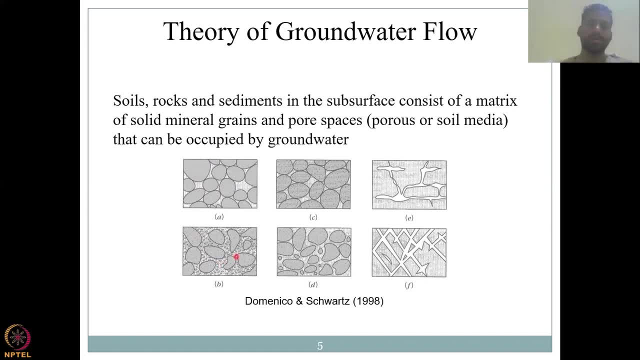 still, you have a good amount of space and that would give you more water to be stored. what is the difference in c in c? the mineral also has its own pore space. so on the rock, on the solid material, you have some dots and spaces in there where 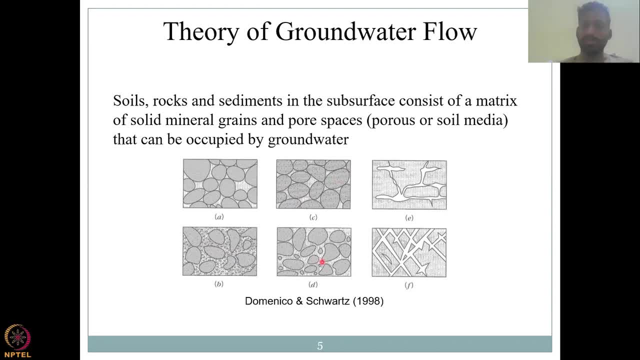 water can be stored. moving on, d is nothing else but the same arrangement, but with more finer particles in between, thereby taking most of the space. e and f are fractured and you can see that you can hold f with a force by using the force factor, f here plus f plus. 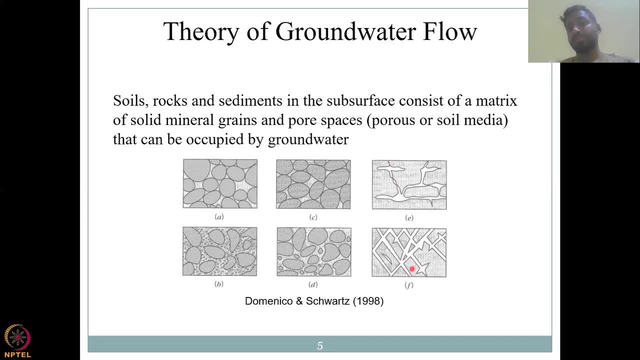 f, and it is because of that it is actually right here. it was in the bit in between those rocks. so let's look at how we can provide the same amount of space that we have in between these two systems. okay, so we have that which is the space in the middle and the one in. 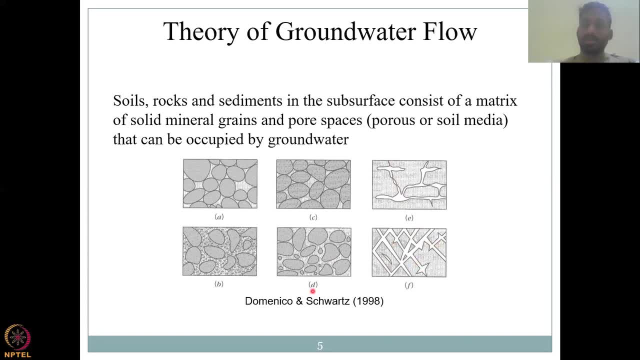 between the two system and the one in between the two species, so we can take the same amount of space in between the two systems. and this is the same type of central structure and this is exactly the same you can also have. you can also see that there is one side. you 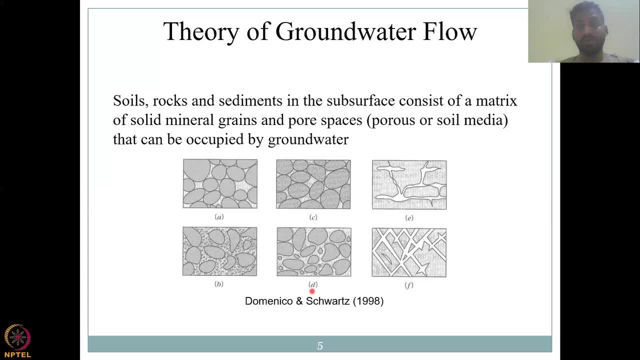 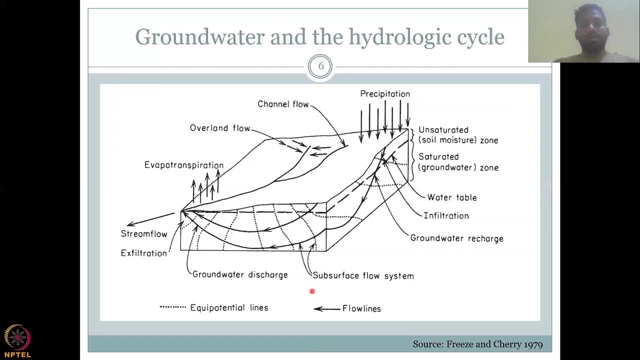 without this space there is no groundwater. So if it is full of solid, there is no place for the water to be going. Moving on, let us see the key formations of groundwater from the hydrological cycle. So, assuming that this is the underground space and it has good 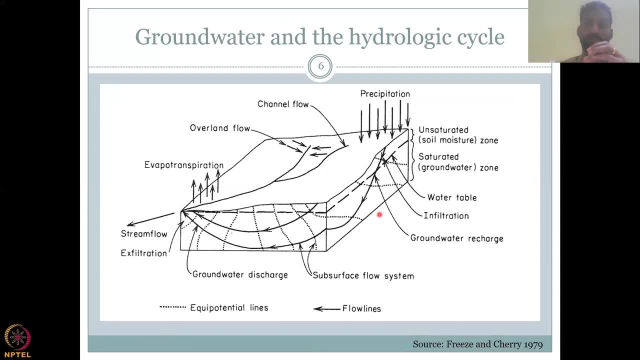 porous space. it has a lot of void, it has a space where groundwater can enter. So that is the assumption when we draw this conceptual diagram. We have precipitation, the key element in bringing water into the system. So first it gets infiltrated, it moves through the 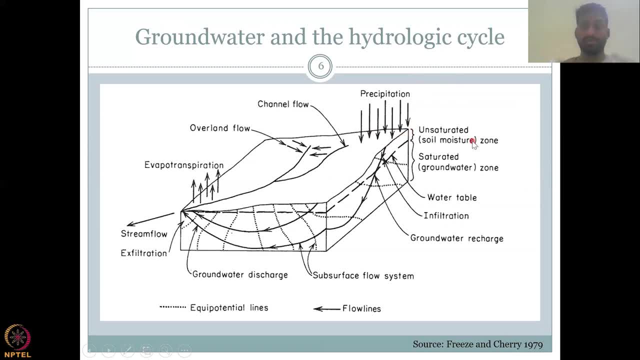 soil zone and soil moisture is increased, which means the soil gets water and the moisture content in the soil increases. So that is the first unsaturated zone. Then water would still continue to move to the saturated zone. We will get into it in a few minutes. 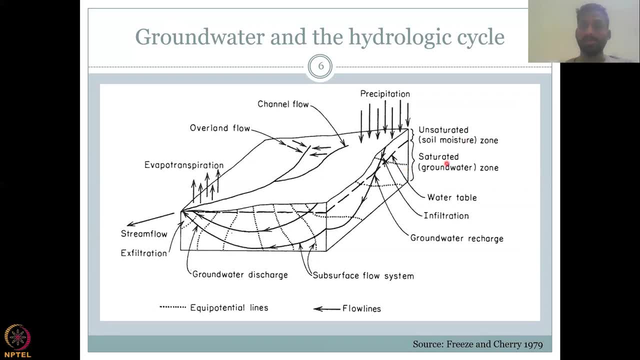 So let us go through a detailed lecture on what is unsaturated and saturated For now. you could look at the top zone and the deeper zones. So precipitation happens first. it goes to the first zone where there is less soil moisture. it will wet the soil and accelerate. 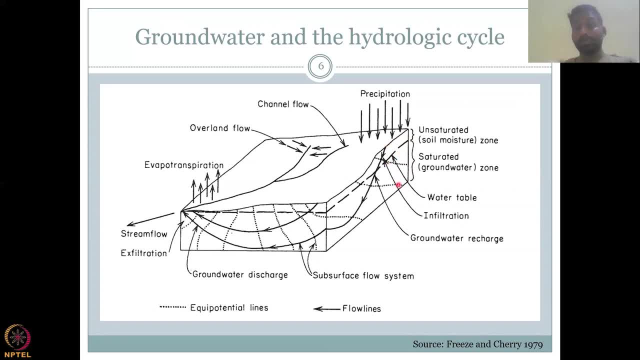 the soil moisture, and then it goes down further. It goes down further until it hits the groundwater through infiltration, and then there is a recharge. So precipitation now gets into the groundwater and then it goes down further. So it goes down further until it hits the groundwater. 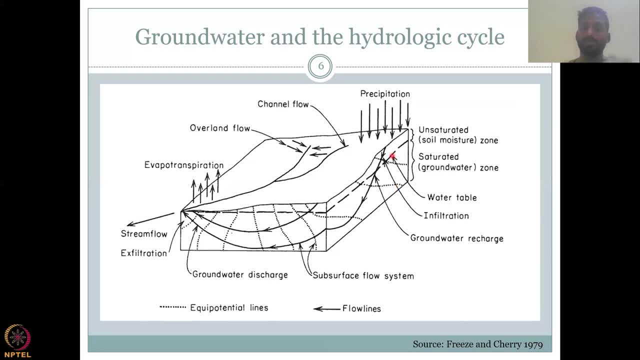 and it recharges the groundwater. Once you have good recharge, it starts to move, It moves and moves until it finds a space in the surface where it can come out and join the surface water body, which is your streamflow. Your channel flow and overland flow are nothing else but precipitation that is converted into. 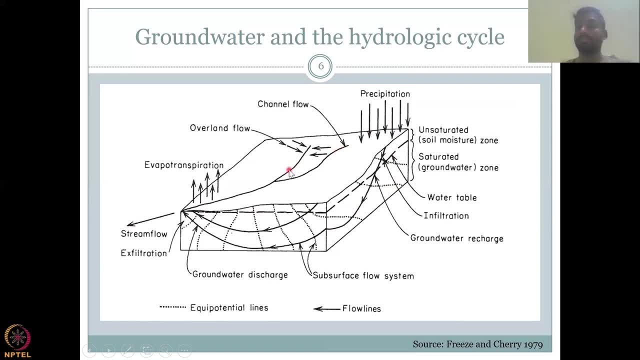 runoff. The sum of the water might be overland flow, It will just hit the land part of it down, but most of it would still go on the surface as runoff, and this runoff can also recharge your groundwater. there are some losses in the system, like evapotranspiration. evapotranspiration is 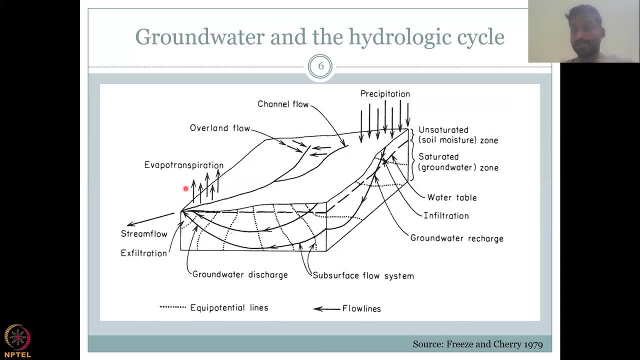 the drying up of water from solid surfaces and also from plants. that transpire, so there is evaporation plus transpiration. we'll just understand that that is a term which is a big loss to the system. it is one of a bigger loss to the system because it takes the water and 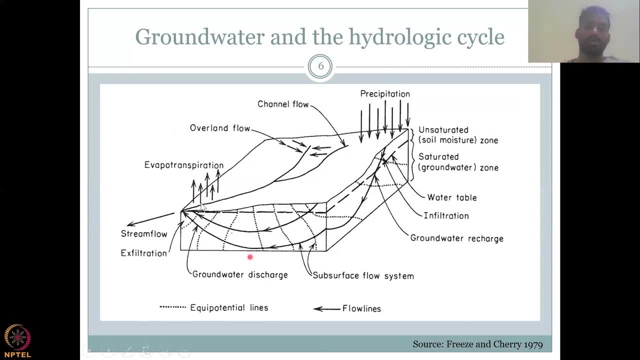 away from the unit of analysis here. the unit of analysis could be a block in a watershed. okay, so if you look at most of these illustrations that i would use, the physics and the theory is still the same, so we'll be using pretty old citations, because they've done a very good job. 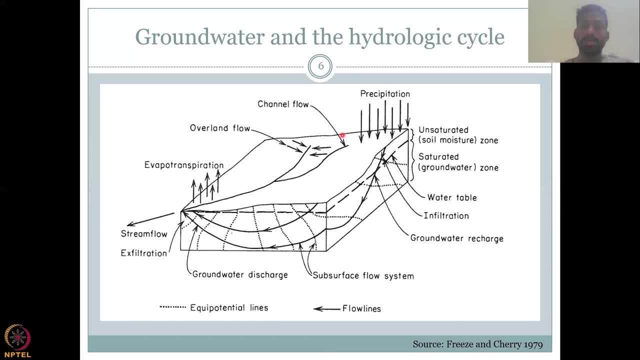 example and for the clearest possible solution. we can use a lot of your suggestions. so what we're going to do here is we're going to be using the example of the charles sutherland, freeze and cherry's 1979 book. groundwater is a very, very well written book and 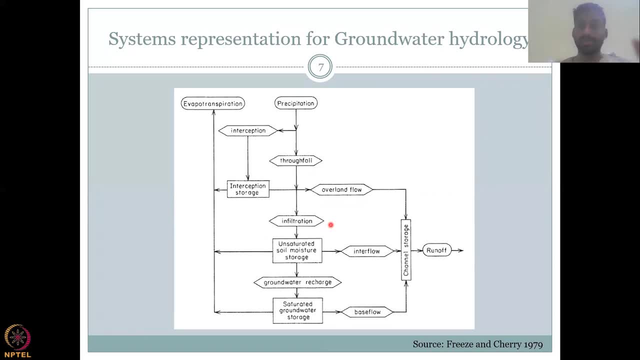 highly used across the world. a lot of policies are written based on that, so most of the lecture would course, but I'll give you the basics from that book. We can also do a systems representation for groundwater hydrology. What is the systems approach? 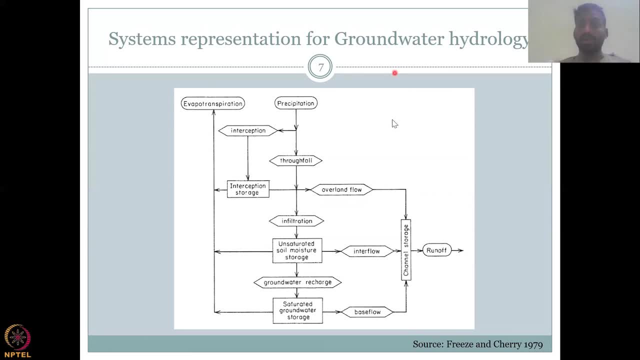 It is a way of showing how, by a flow diagram, each components give rise to a different component, and where there is storage losses in the system. okay, So we start with precipitation coming into the system. Okay, our system is the unit of analysis. 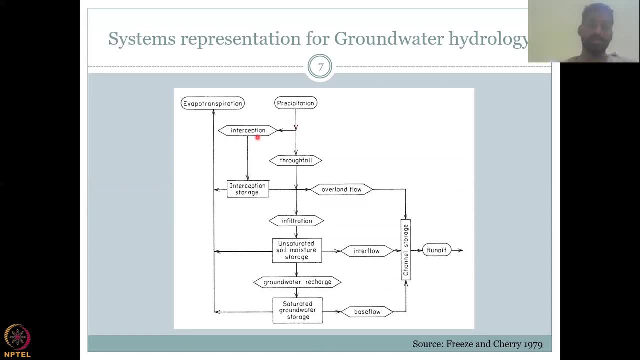 Part of the water is getting intercepted. Interception means you're stopping the water right. So you're stopping the water through what Trees plants? Think about the atmosphere. You have a cloud and then rainfall occurs. The first thing it hits is not the land, but your trees. 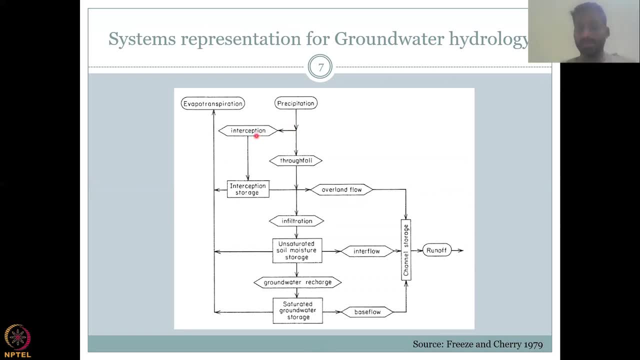 your trees branches and then it comes down, So that is called interception. There is some water stored in interception. The remaining water goes out. That's evapotranspiration. Remember I told a word about evapotranspiration in the previous slide. 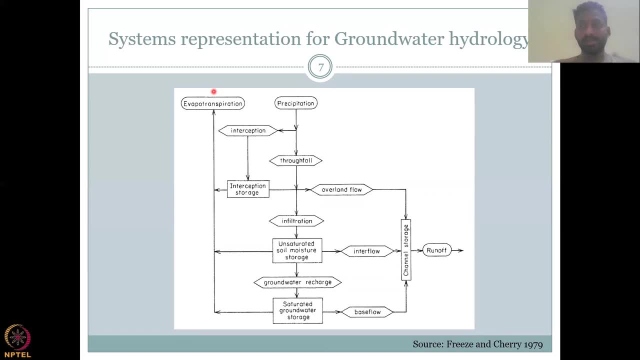 It is basically a loss of water from the system due to evaporation and transpiration. Evaporation means drying up. You put water on a solid surface after some time due to heat and evaporate. it evaporates right Because evaporation drives up. 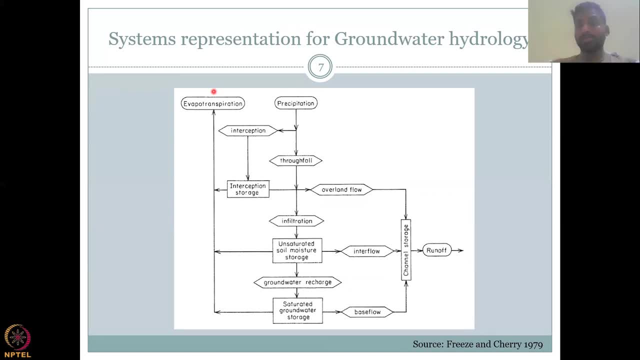 Transpiration is the fact when plants take water to the roots, to up to the shoot, up to the plant leaf area, and then it transpires it out, It converts it into water vapor, It mixes into the water vapor, So all this is as a vapor, evapotranspiration. 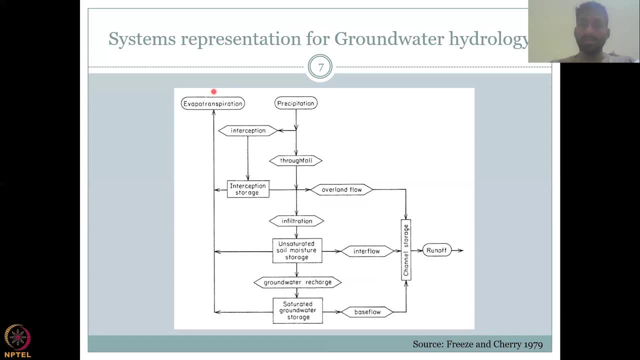 is a vapor state, okay, It is a gaseous state, not liquid. Precipitation is a liquid, interception is a liquid, storage is a liquid. Then you have- okay, you have evapotranspiration, but for now you please understand that it is a loss to the system. 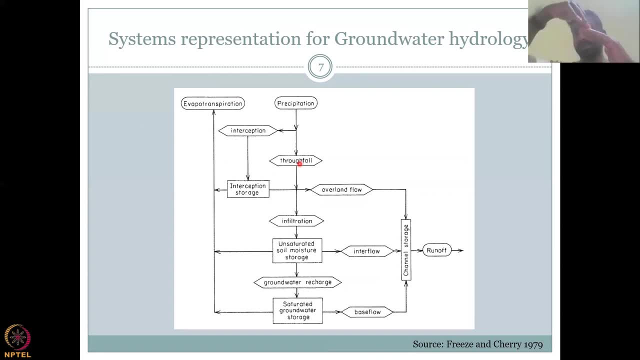 moving on. so the plants and trees that are stopping the water goes into interception. but there are some water that can still pass through, okay, and that is called through fall. so water will pass through the system and first thing it will hit is the land. once your rainfall. 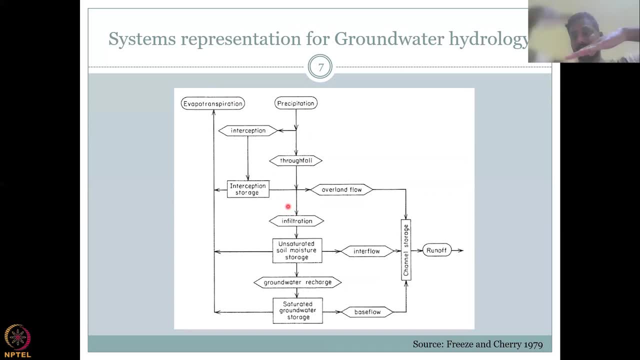 hits the land, part of the water will go as runoff. it'll just slide on the top as runoff and that is called overland flow. there are different terms used for runoff. there's overland flow water and flow, subsurface flow, etc. etc. here it is given overland flow. okay, so it is runoff. 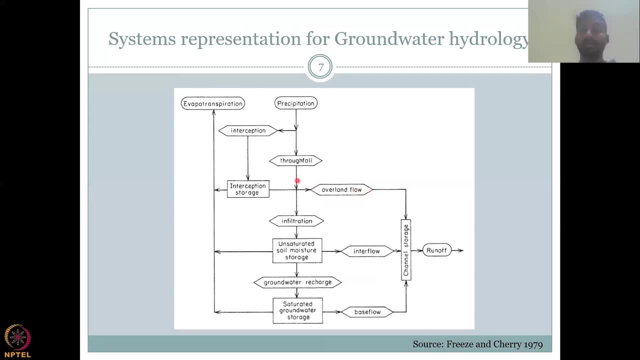 or overland flow and then the remaining water can go in as infiltration. so i said: rainfall hits, this is your land. part of it gets infiltrated and goes through, but most of it would run through as runoff. it will go like this due to the slow gravity etc. once it goes into infiltration, the first zone it sees is the unsaturated zone. 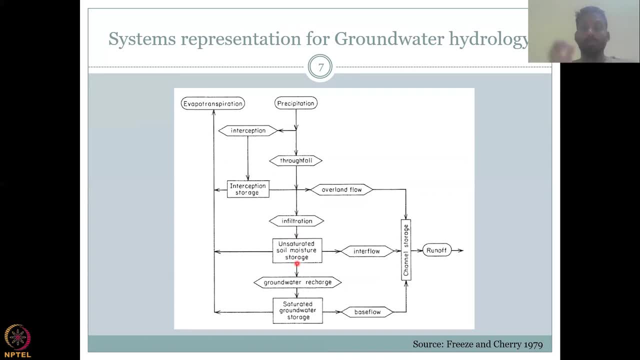 unsaturated means not full with water, so the water will enter the unsaturated zone and improve the storage and part of it goes to plants or evapotranspiration. so, since it is the first zone, there is a lot of roots and the roots can eventually take water and evaporate, transpire. 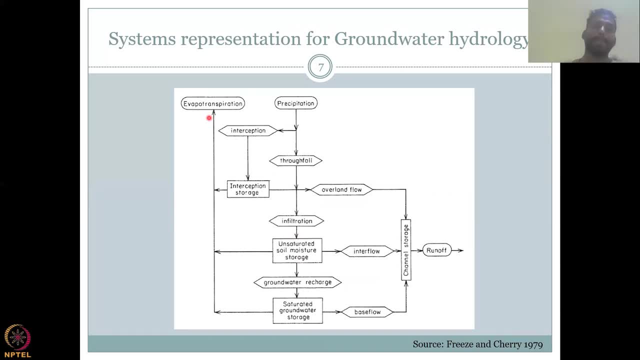 contribute to evapotranspiration. then you have the overland flow that goes into the channel storage, which is your river, channel, stream, channel, canals etc. and part of your unsaturated zone groundwater can go as interflow. interflow means between the overland and the bottom aquifer. 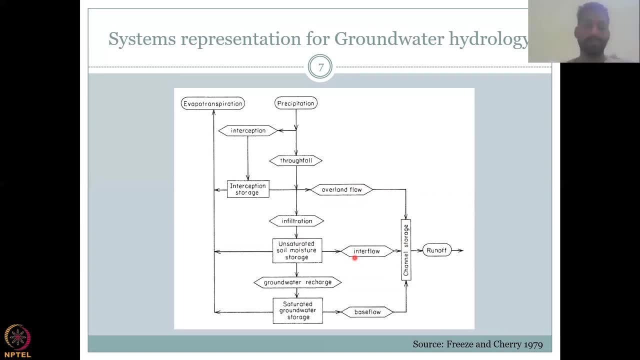 some water can go as flow, the subsurface flow. so after the unsaturated zone, water is taken up by the plants. still some water moves down. you can see all of the arrows moving down because of gravity. so this is your atmosphere, this is your trees and this is your zero land level: the land at zero, and then water. 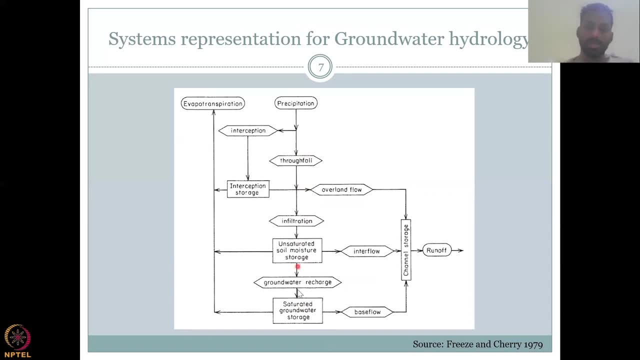 moves down, still because of gravity. so once it comes down below the unsaturated zone it enters the groundwater recharge area. so water starts to recharge and the recharge would give more water to the saturated groundwater storage, which is a unit where water is full already and when you put more. 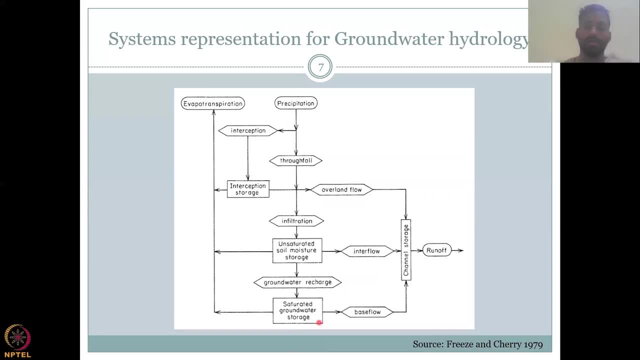 water. the level of the water rises and from here still plants and trees can take the water as and transpire. so the transpiration is still happening through these lines of unsaturated and stored saturated water and part of the saturated water goes as base flow. a base flow is part of the groundwater. 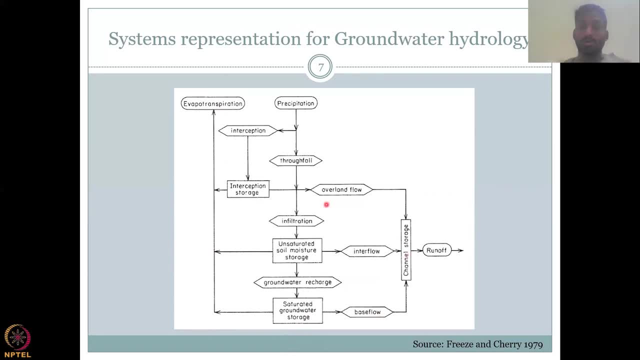 that goes back into the channels. so, if you see here, your overland flow, which is your rainfall, goes on the top of the surface into the rivers, and then there is some water which would infiltrate, slowly infiltrate, and part of that goes as into the stream, as interflow, but there's another water. 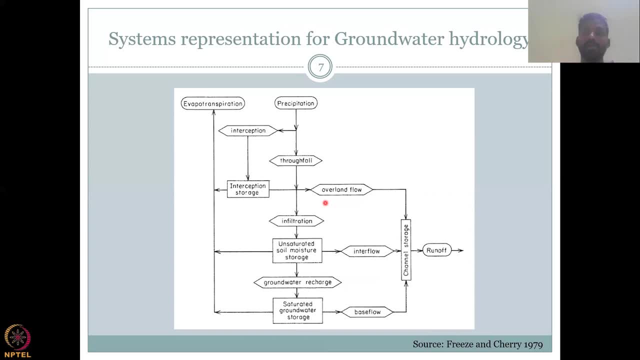 which goes deeper and deeper, deeper into the groundwater and then it goes back into the channels and from there it goes into the channel storage and then it all combines into one unit called runoff, and the runoff can be your stream, your river, and it can eventually join lakes, ponds. 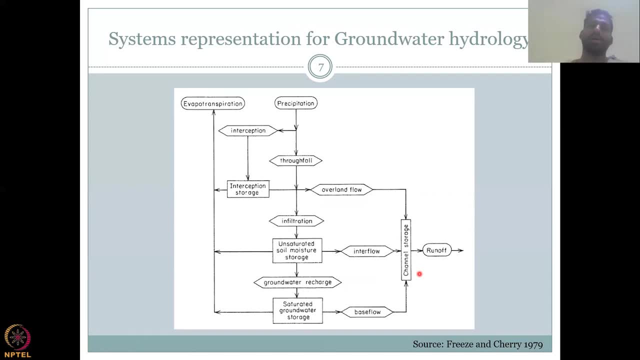 ocean or seas. okay, so that it closes the hydrological cycle again. so this is a very simplified representation of the groundwater hydrology, how groundwater forms from precipitation and then goes through all these different compartments. it is also important to note that the contribution of each variable depends on where you take the data from. 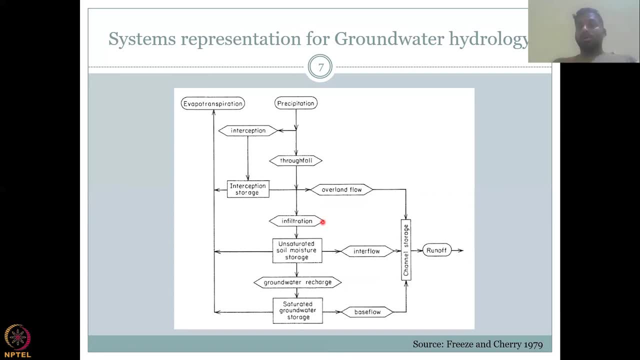 for example, if you're desert, there's more evaporation because of the tremendous heat, and if there are water bodies, there's more water stored on the surface. so those kind of things. so you have to understand where to use this explicitly, but it gives you a very fair, broad idea about how water moves. what are the major? 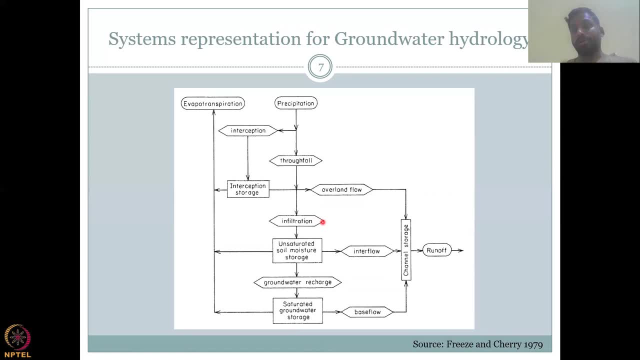 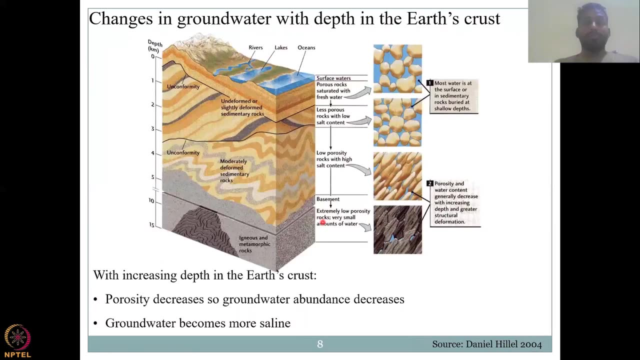 components and then how it comes back into runoff, into the hydrological cycle and does the cycle again moving on. we also should understand that when you go down deeper and deeper into the river or into the solid zone, sediment's, sand, etc. these pore space, the space where water 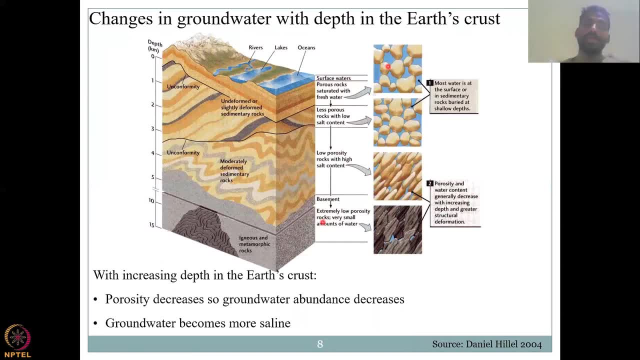 is stored, which is the fundamental for groundwater hydrology, is reduced. okay, so you have the surface, you have all the water coming in and water moves down groundwater system and then it saturates, which means it gives water into the space and then, if it goes more down, you see that the number of spaces 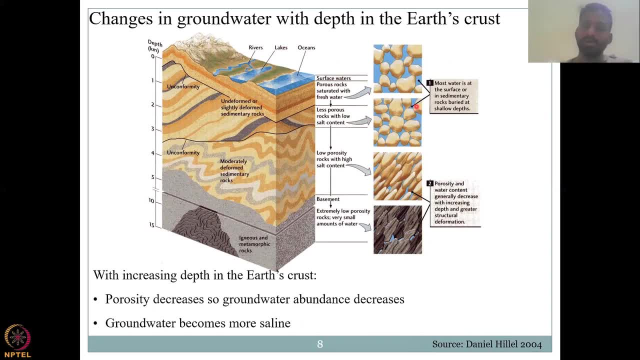 is reducing, the volume of space is reducing and that is because the final sediments would clog the space. if you go down further, the sediments would have more structure, more solid, rigid structure. it will not be disintegrated, as on the above and by the. 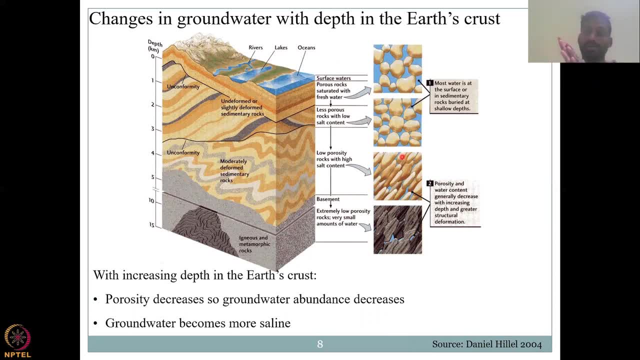 means of when it is more structured or platy or something. rocks do not have much space in between, so you can see that the space has decreased when you go down into the earth's crust and then, finally, you come to the bedrock region, where there's very less groundwater potential because the space is 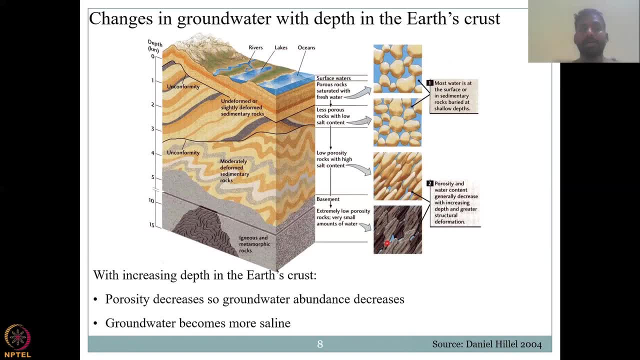 less so. when someone talks about groundwater potential, it is the potential of the solid under the ground to actually store the water. how much space is there? if the space is very less, then the potential is you very limited. okay, here you see the potential decreasing from the top to the bottom, and the bottom has the least. 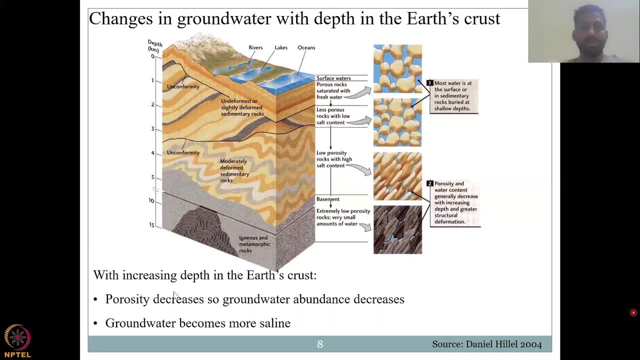 potential. so what do we have here? with increasing depth in the earth's crust from the top, you're decreasing in the depth, porosity decreases, the space between the solid materials and the sediments and etc. decreases, so groundwater occurrence and abundance decreases. therefore, larger surface is in less module and the surface being thinner because the way water departments 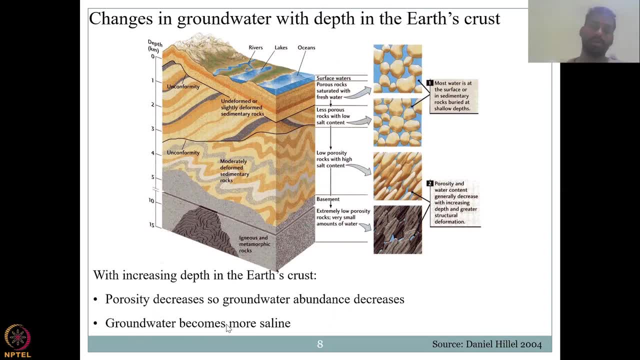 re applicable. more importantly, groundwater becomes more saline if you go down deeper and deeper because the water is with old, old rocks that has that are not disintegrated, and once the water starts to disintegrate or weather the rock, then some salts from the rock would be mixed with the 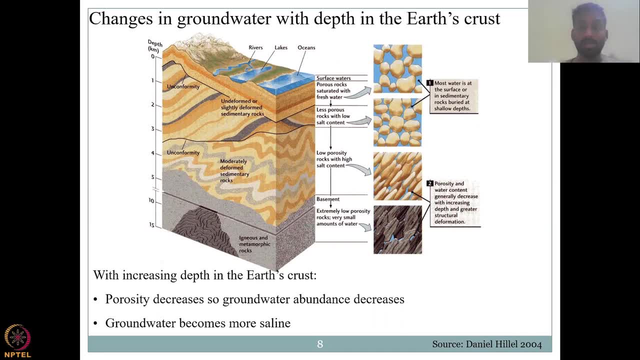 water and becomes selling. saline doesn't mean salty tasty alone, but saline means with salt and itぉn finds that the water gets cover tua place of saline, that means it plays for the environment value. but if that is accumulated inside ox or other water sources, and then itlo Punkt이트 Christians. 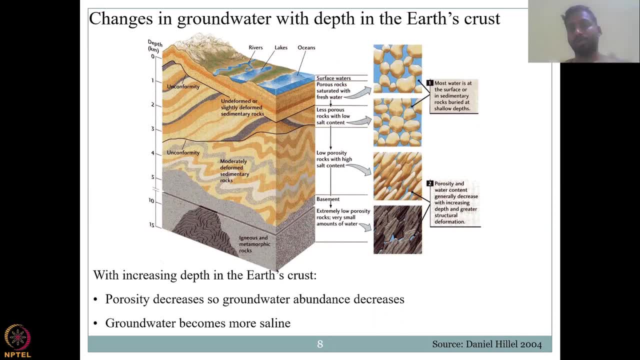 size, attennity, et cetera, Champion of our internal balance between salt and water. but it's also like great and, but it's just classic, so we say no digression, it is fine. france Islamic organization by nature in a with salt, and salt is from the rock mineral here. it's not the ocean salt that we're talking about. 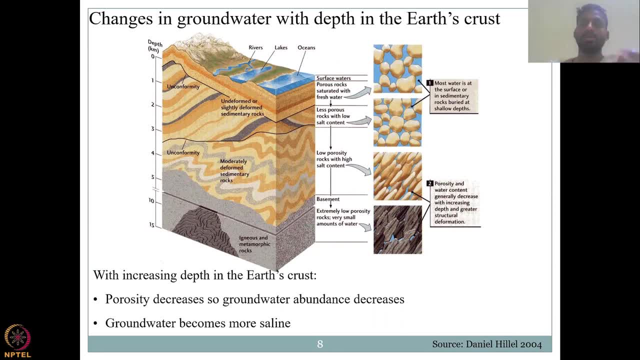 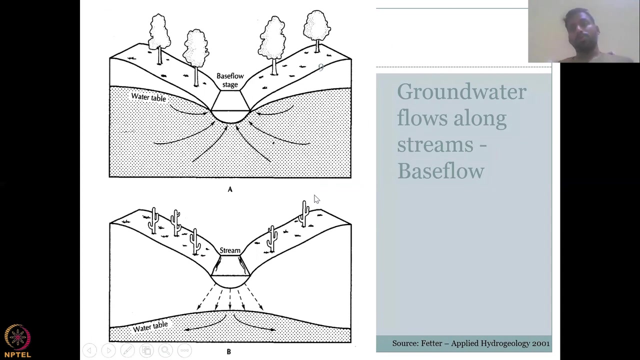 it is a mineral, the rock will have some particles that will enter us as salts. so the take home from this message this image is: groundwater is important and it comes from the surface to the bedrock. this is the rock where no groundwater is available, but as we go deeper and deeper you will lose your groundwater occurrence. 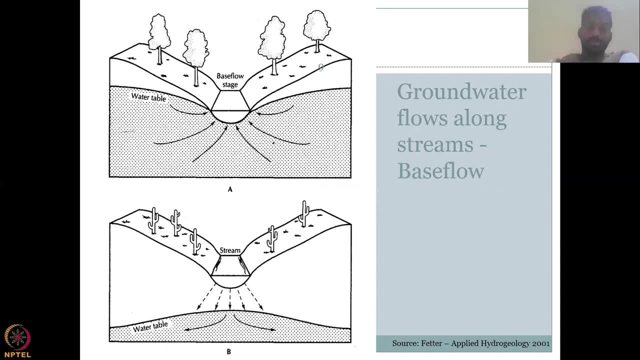 it's also important to see ground water flow along streams. so this is a forest- you can see the trees, which is different from the bottom one, which is deserts. you have cactus here in B, whereas in A you have trees. so if you have water coming on the top as rainfall, it can get into the ground and from the ground 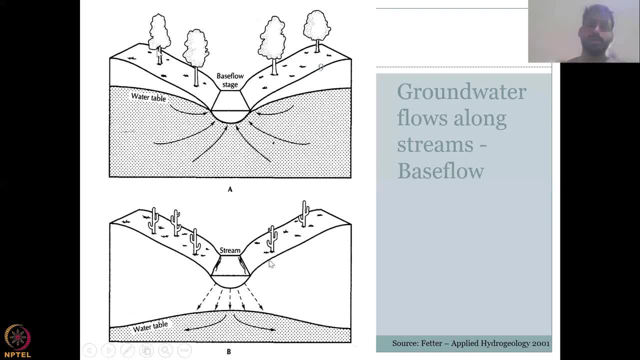 it can come back into the river. So this phenomena of groundwater providing water to the surface- okay- is an input to the stream and thereby the stream is gaining, the stream is gaining water, whereas in a desert system, for example, water is available in the stream, maybe, maybe a canal was. 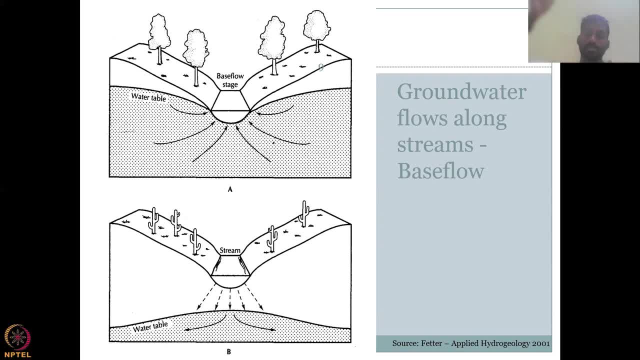 brought or big rainfall is there. it is. it is concentrating the water and flowing through a river. a big channel is there and that channel will give water down to the groundwater table, because the groundwater is lower than the stream level. here, if you see, the stream level is lower. 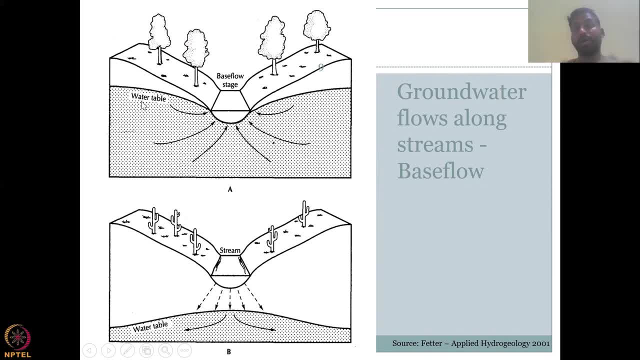 than the groundwater. so the groundwater gives water from the high potential to low potential. so groundwater table is high potential. it goes to the low potential, which is stream flow here in diagram b. now, if you do the potential energy for this, the groundwater is at a low potential compared to the stream and so the 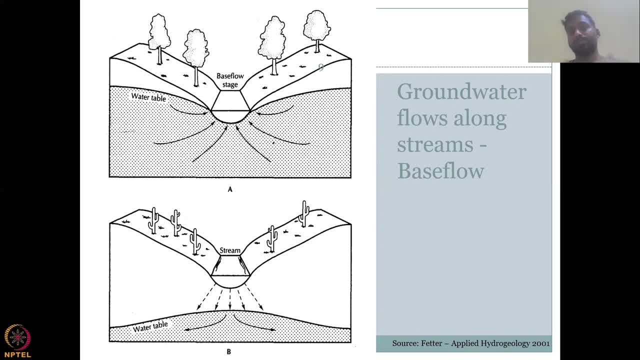 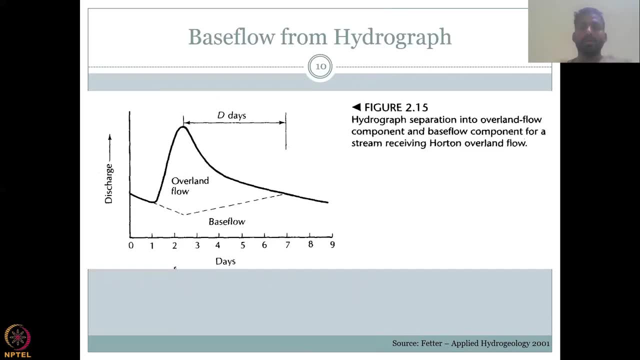 stream can give water to the groundwater. always, water flows from high potential to low potential, so this can also be understood from a hydrograph. what is a hydrograph? a hydrograph is the graph with x-axis having the time and your discharge on the y-axis. it's basically a time representation of your discharge of your river. okay, so if you 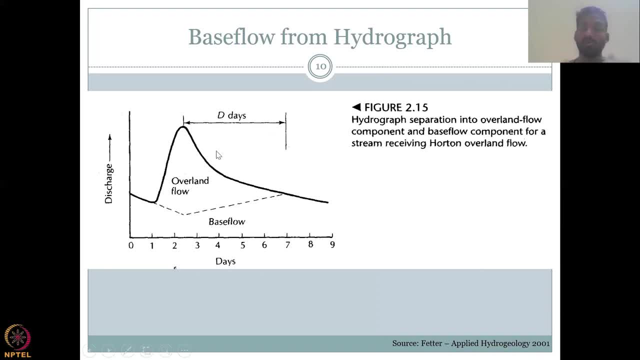 could see here. when there is rainfall, then the stream flow picks up, but when there is no stream flow happening and no rainfall, then it is not a perennial stream, it is a seasonal stream. but in a perennial stream, what happens when there is no rainfall? still you see some flow, like, for example: 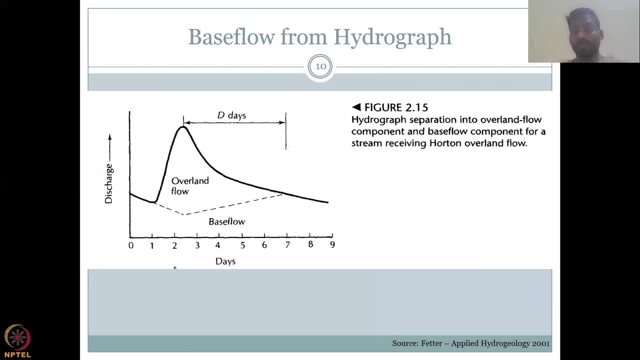 Ganges, Cauvery, etc. have flow in their stream to the ground. but when they are in a perennial stream, flows for a long time right and what happens actually is part of the groundwater gives in into your stream flow and that is called base flow and you could easily calculate it by looking at. 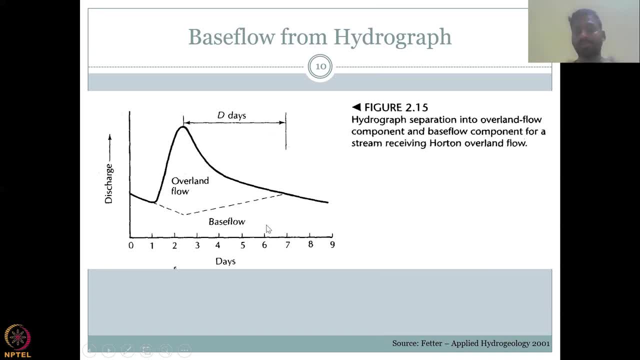 the discharge before the rainfall and after some days from the rainfall. so before the rainfall. so exactly here, the second day, maybe the rainfall started, but before that you still have river water flowing and that is because of base flow contribution, which is groundwater giving water into the river. and after the rainfall stops, still after some days, your groundwater can come back and 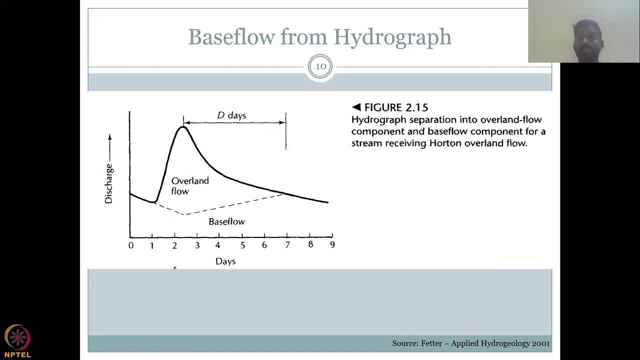 give water more to the system. so to understand this from the previous diagrams: in a groundwater hydrology water is first taken from the surface through precipitation, infiltration and percolation. then water moves through different compartments and exits back into the stream and that could be called as a base flow. so base flow is nothing but the groundwater contribution to stream flow.